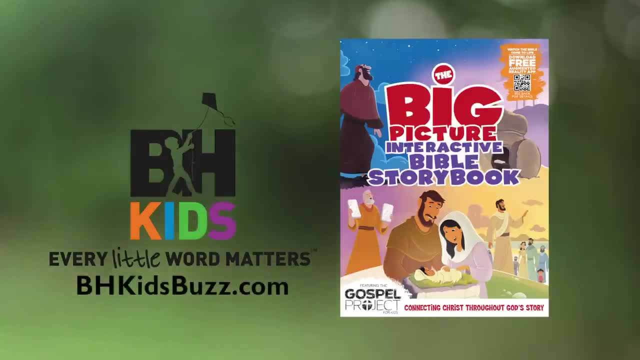 Visit us online at bhkidsbuzzcom. B&H Kids AR. 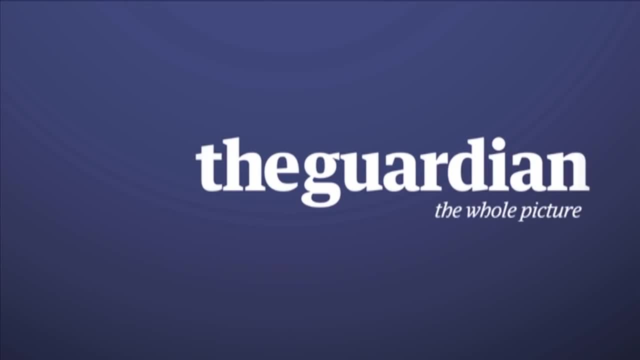 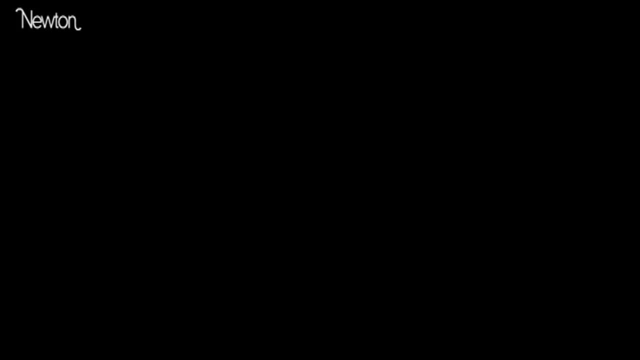 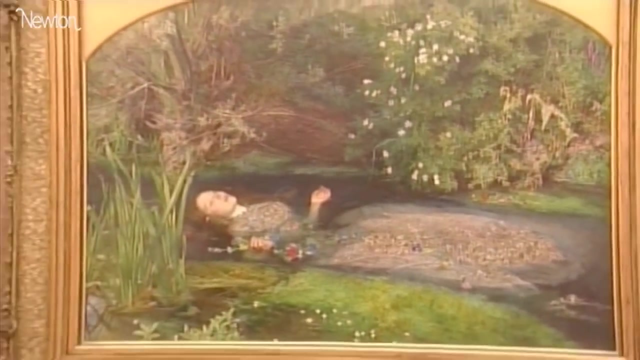 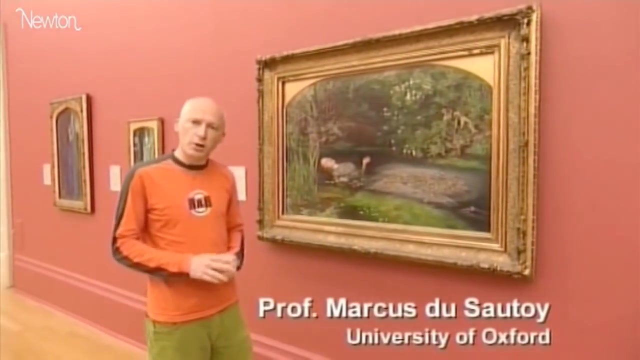 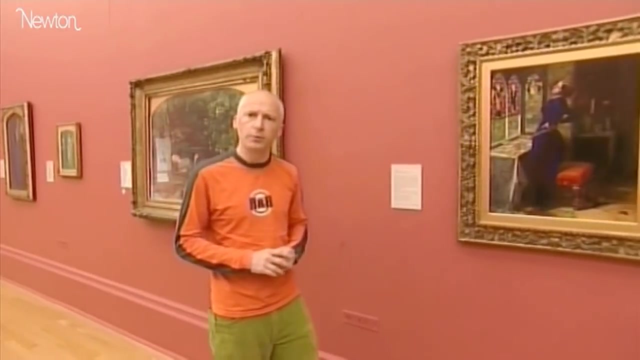 Beautiful, isn't it? This painting was regarded in its day as one of the most accurate and elaborate studies of nature ever made. In my mind, an equation can be just as beautiful. Instead of paint and canvas, a mathematician uses numbers and equations to depict everything. 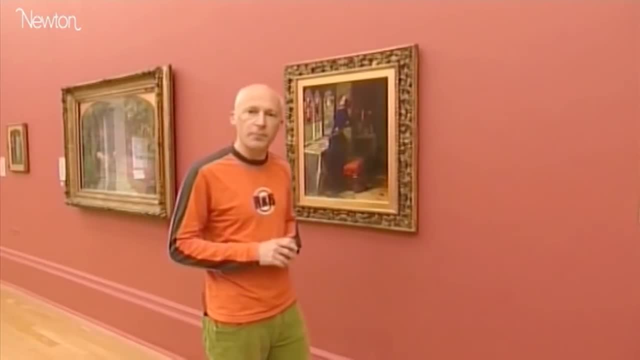 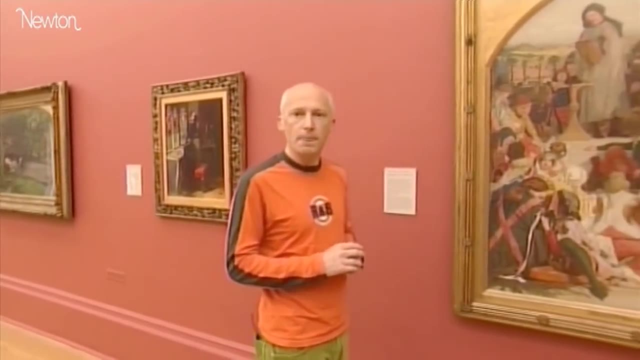 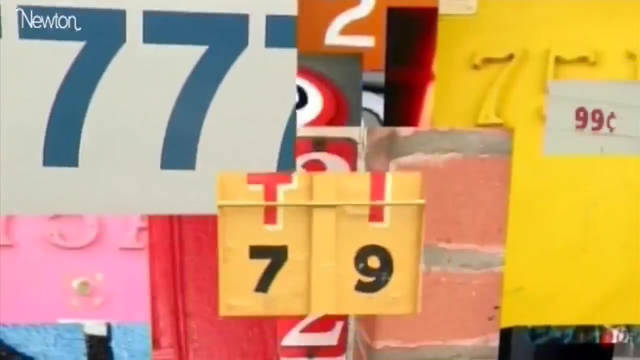 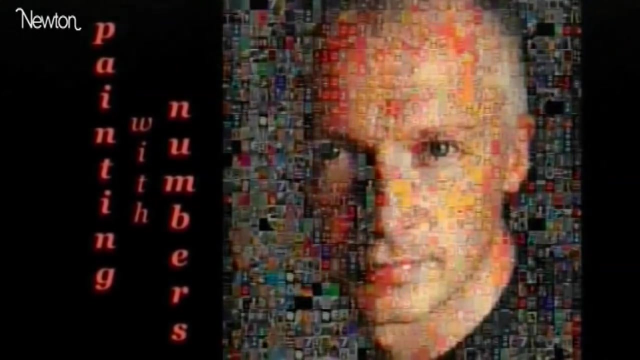 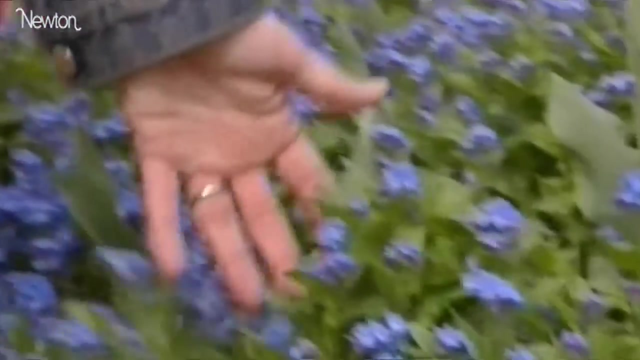 from the movement of atoms to the formation of galaxies. Mathematics can be used to view the world in a way that is as breathtaking as a Van Gogh, Monet or Renoir. The universe is literally painted with numbers. Have you ever counted the number of petals on a flower, Given the variety of different? 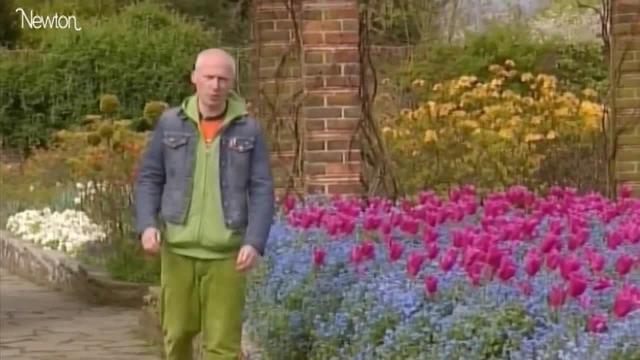 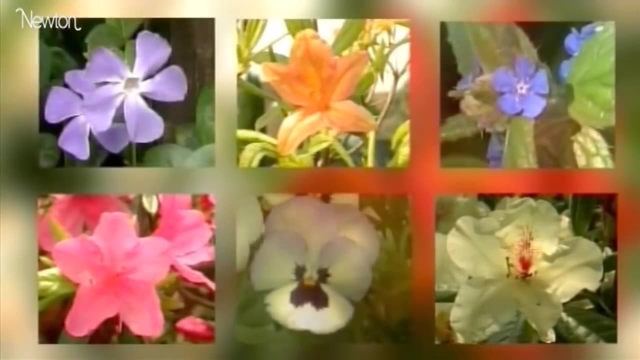 flowers in the garden. you might think that any number of petals was possible, But it turns out that many flowers like just five petals, And if it isn't five then they seem to favour other numbers like eight, three, four, five, six, seven, eight, nine, ten. 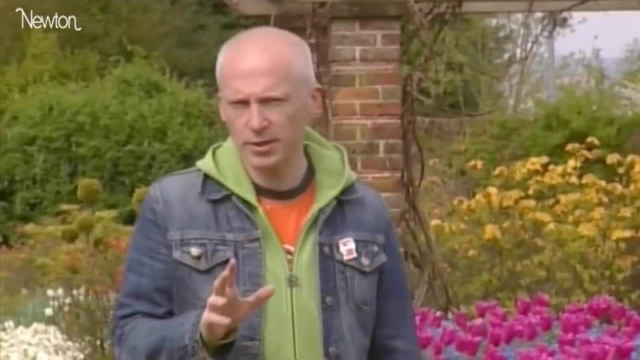 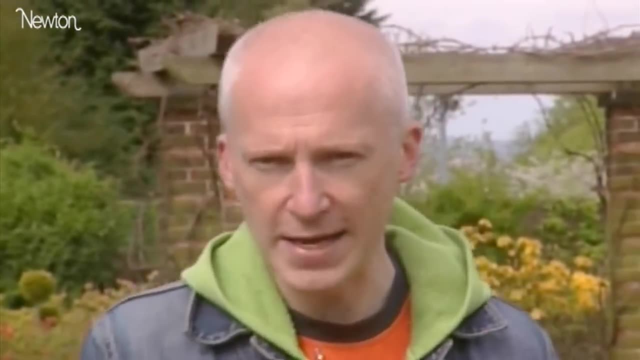 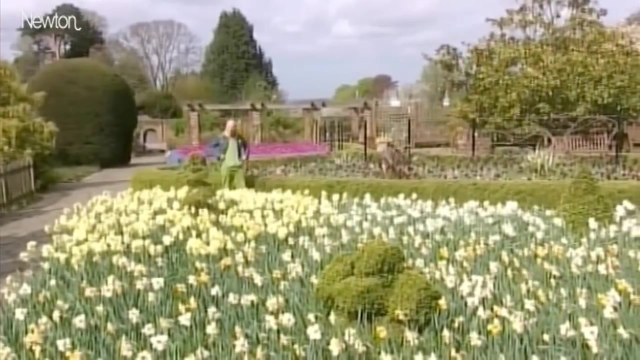 thirteen, twenty-one. Perhaps you can see a connection between all of these numbers. You get each number by adding the two previous numbers together. So, for example, eight plus thirteen gives you twenty-one. These are called the Fibonacci numbers and they're nature's favourite numbers, You find. 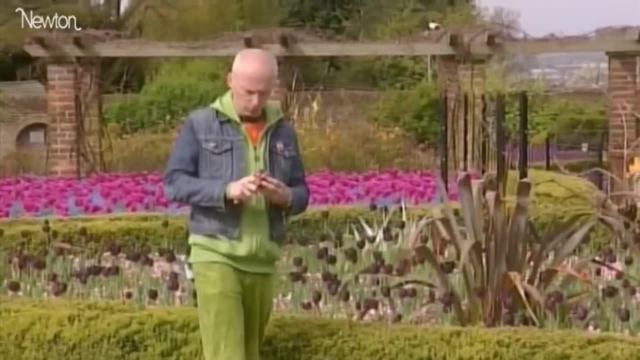 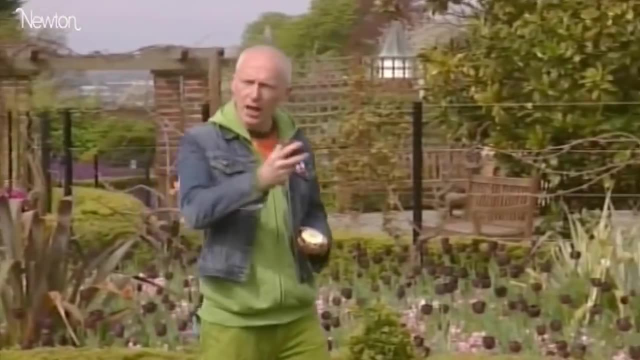 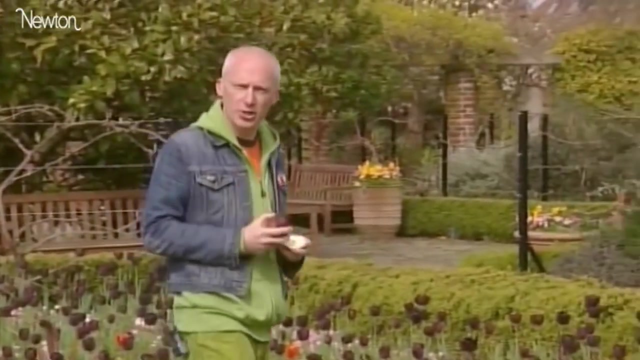 them all over the natural world. Take an apple, for example. Cut it in half and you'll find five seeds at the centre of the apple. Count the number of spirals on a pinecone Or on a pineapple And you'll find two sequential Fibonacci numbers, Say eight and thirteen. 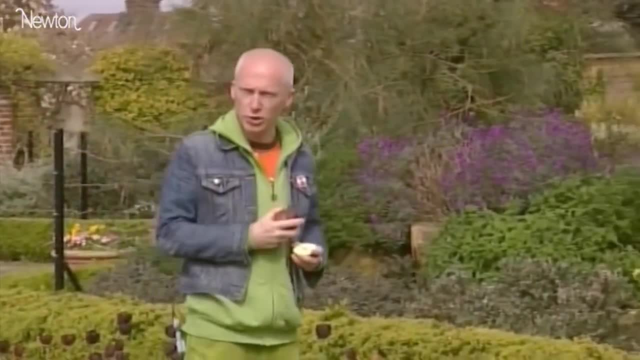 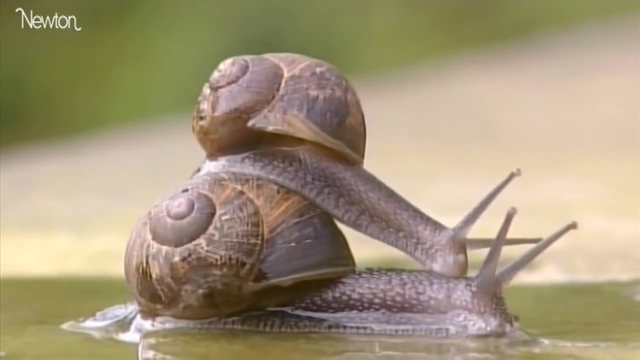 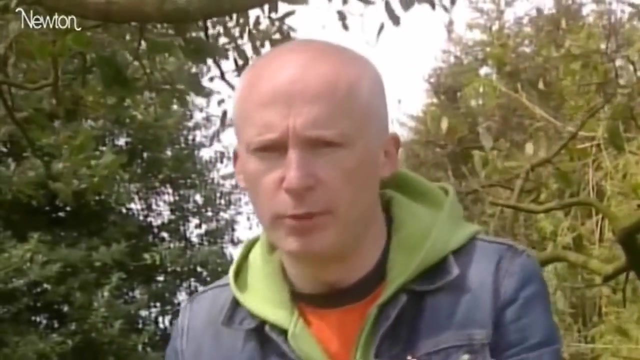 Plant growth seems to obey mathematical rules. But it's not just flowers that like these remarkable numbers. Snails build their shells in very much the same way as the Fibonacci numbers are built. A baby snail starts off with a tiny shell, Kind of one by one square.